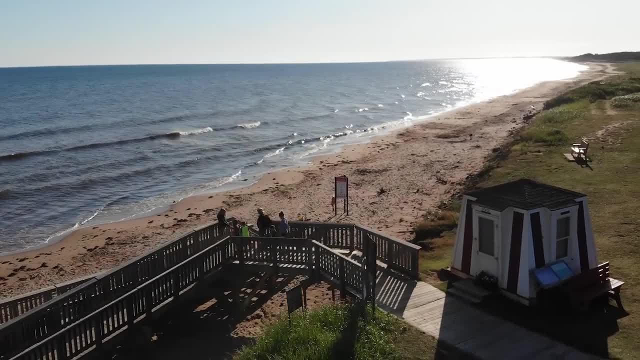 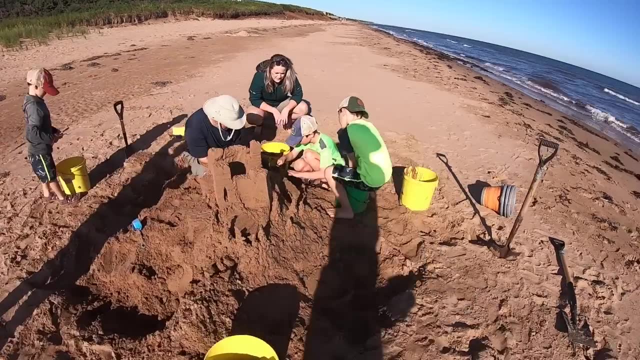 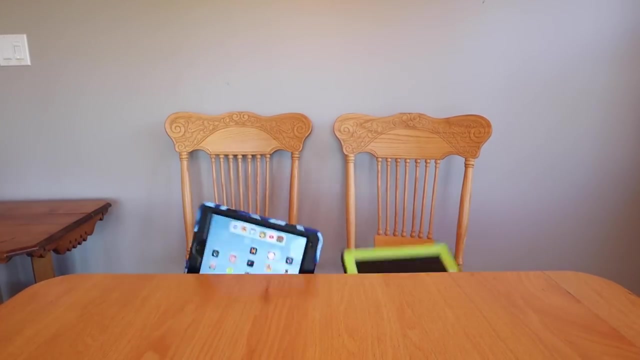 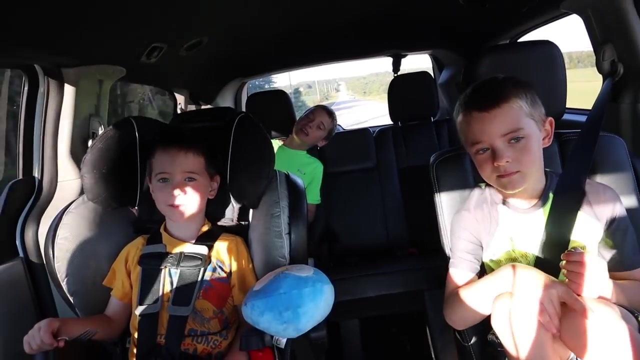 I'm Jessica from Parks, Canada. Today you'll be working with our sand castle expert, Maurice, Building a really epic real life sand castle. See you in a minute. How y'all do this morning? Good, Y'all ready to build some sand castles, Yeah. 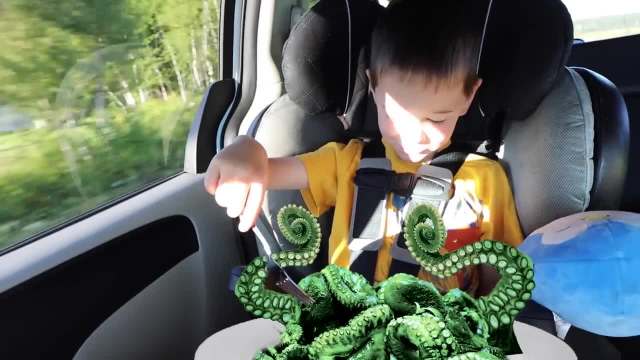 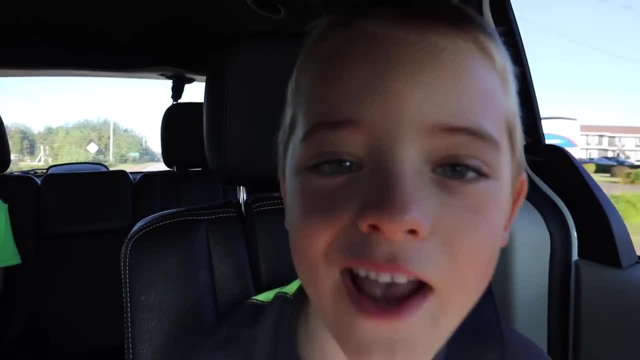 Oh, how's your breakfast? Yeah, I'm ready. You ready to build some sand castles? Yeah, I'm ready. Whoa, we are early. There's nobody here. I think we are in for a fantastic day, Awesome. 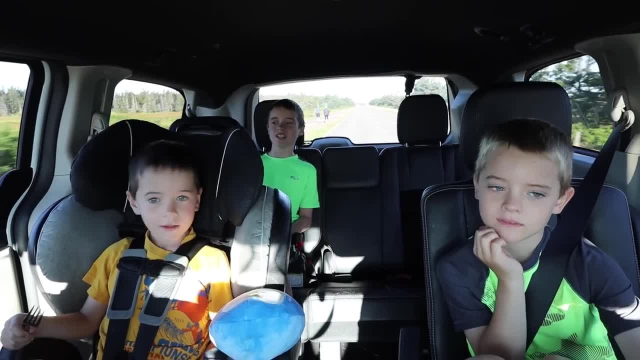 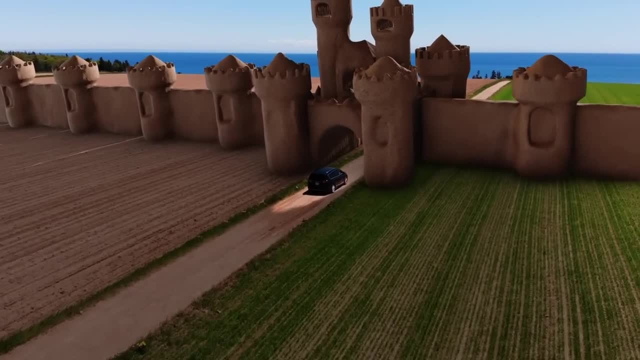 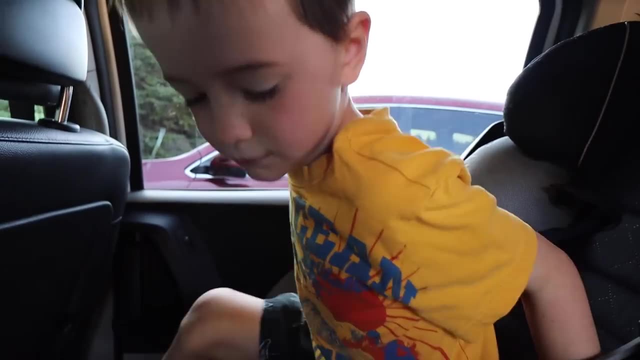 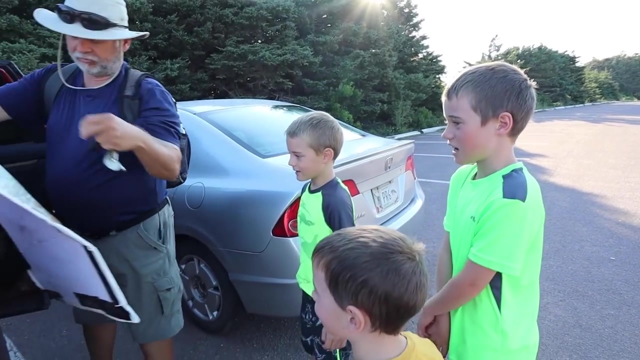 How high is our sand castle going to be? Like as high as this van? No life size. Yeah, And we're here. It's time to meet Maurice Maurice from Experience PEI. He is a professional sand castle builder, Wow. 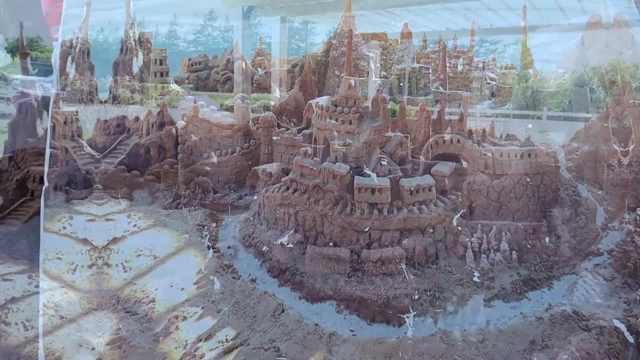 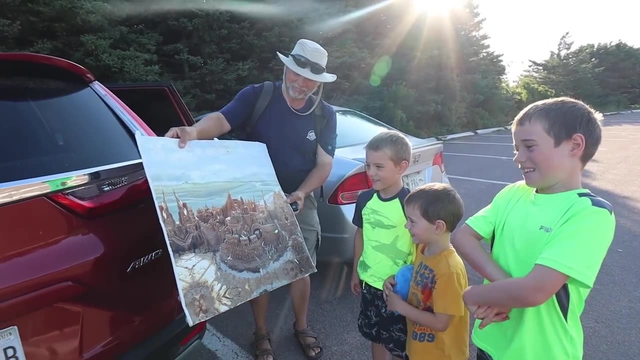 That's cool. What, Oh amazing Um will ours be that big, Biggles, Biggles, Biggles, Biggles, Biggles? Okay, Let's grab our gear and head to the beach. And what a beach it is. 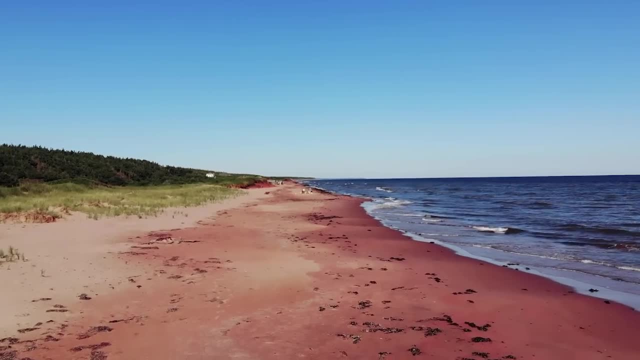 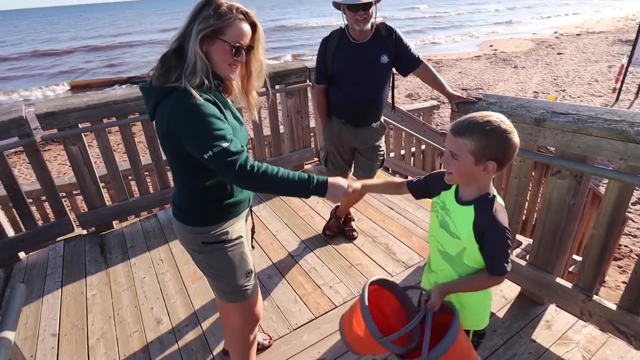 With its famous red sand Perfect for making sand castles. And what a beach. it is Perfect for making sand castles And we're the only ones here. Oh, and Jessica, Nice to meet you. This is River Hi River. 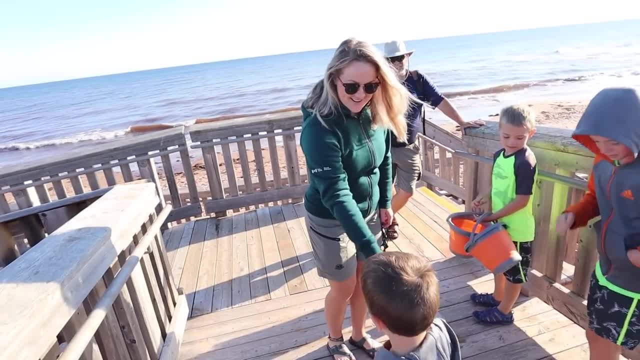 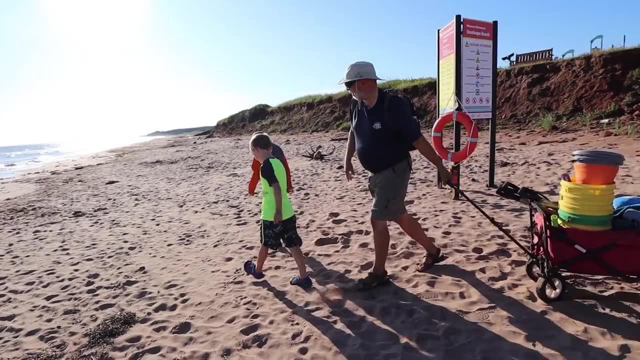 Nice to meet you. And the Archer shake a hand. Hi, Archer, Nice to meet you. I'm Lupin. Oh Okay, team Great. so we'll go down this way, guys, Maurice has an awesome cart full of tools. 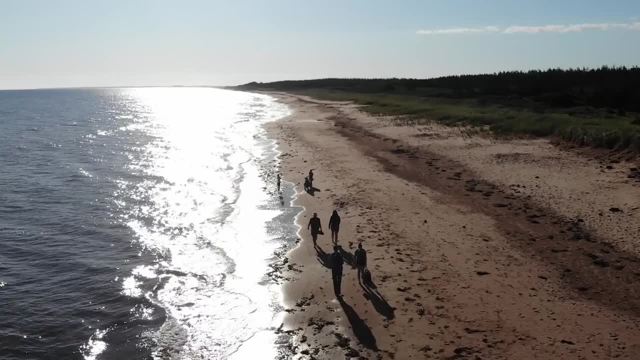 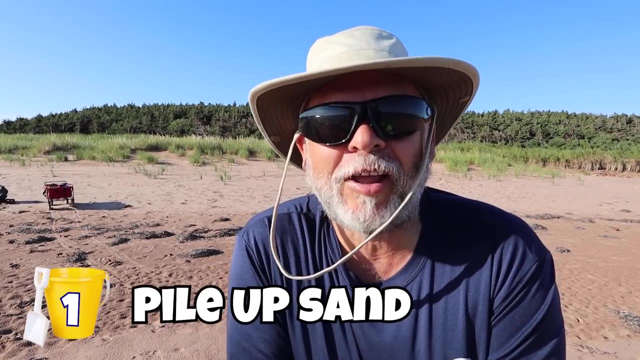 We'll help him take it down the beach, Where Maurice will show us some of his sand castle building secrets. The first thing we're going to do is pile the sand up. Hey guys, it's me. Archer, Are you ready to get building? 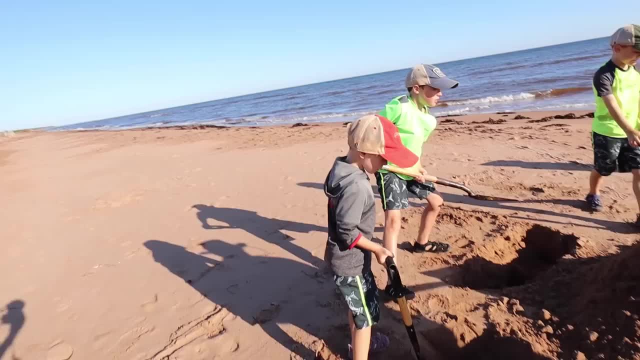 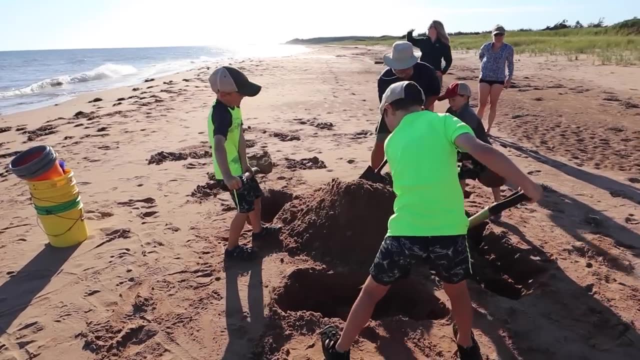 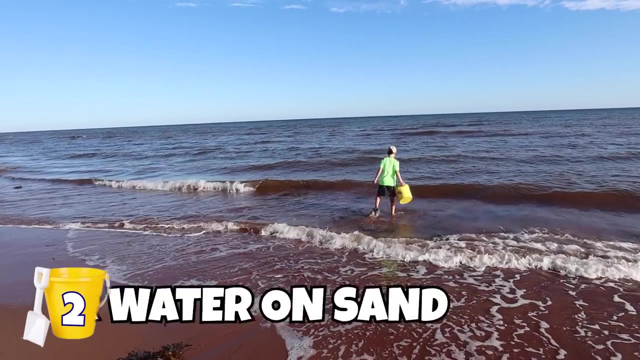 Archer, are you going to sleep in the castle tonight? Yeah, Only for me. See how crumbly it is. So we're going to get rid of that crumble. So we got to pour water right on it. Okay, step two. 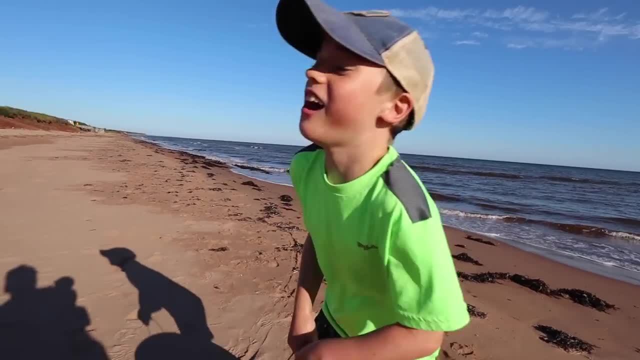 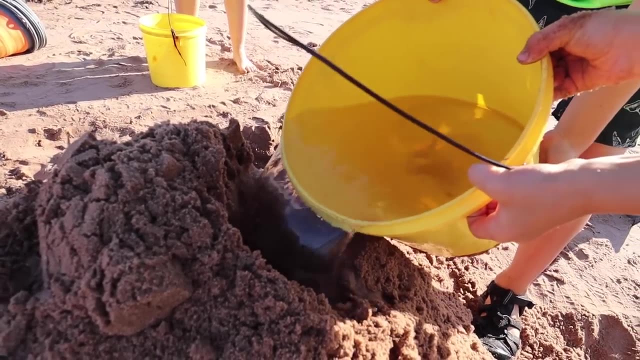 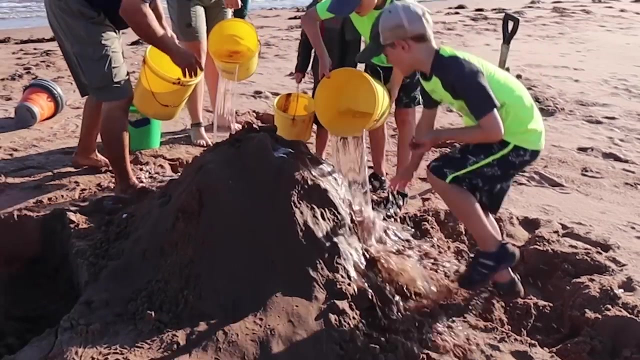 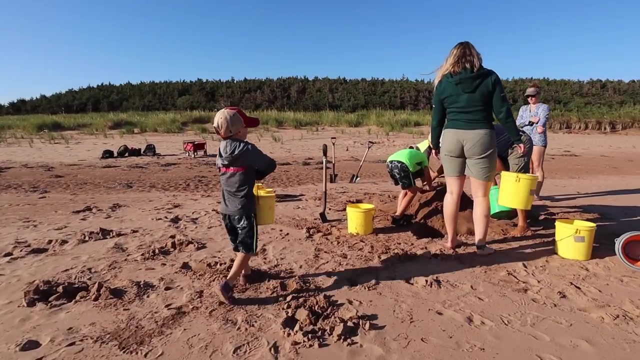 Pour water on the sand. It's heavy. Come and pour it in this hole In the hole, And then you see all this. There's an old barrel over there, Just get it wet. Whoo Archer's got some more water. 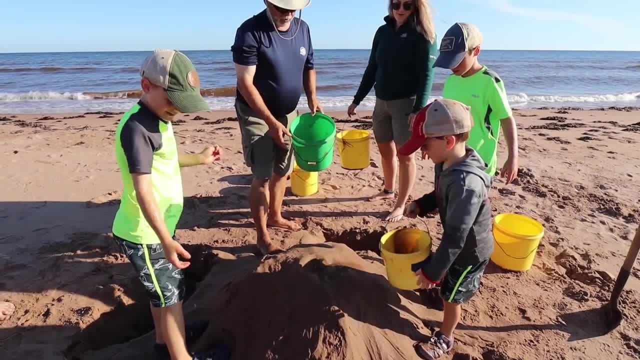 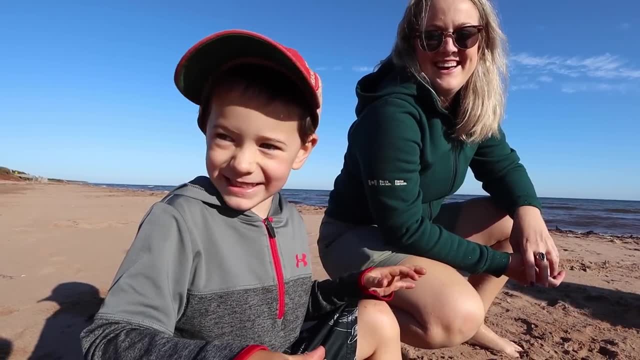 Whoo, There we go. I think that's enough water there. How you doing, Archer? Good, This is the best day ever. Well, come over here and then I'm going to show you how to build up And put it in the bucket. 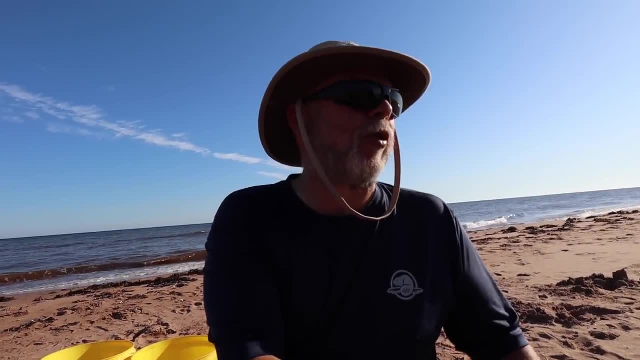 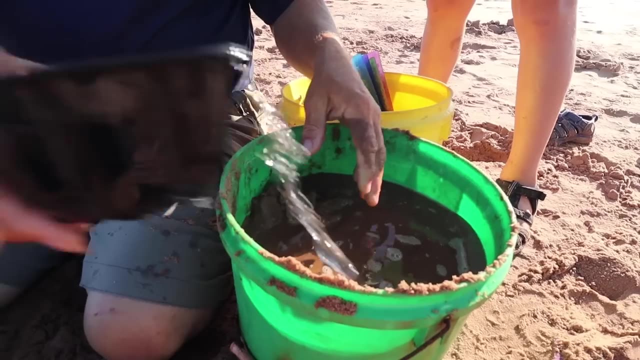 Okay, so we're mixing the water with the sand to make perfect mud. Step three: Mix the perfect mud. The mixture has to be just right. I always have to have water on top of the mud. There's always a skim of water. 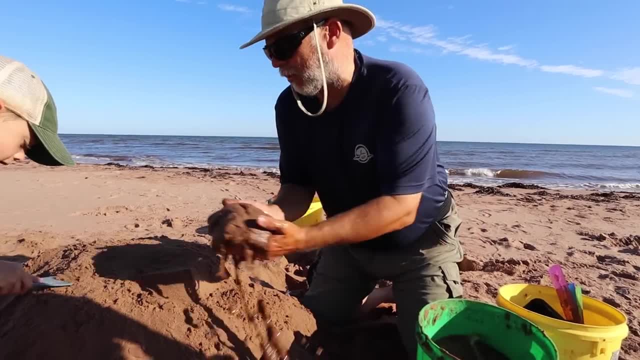 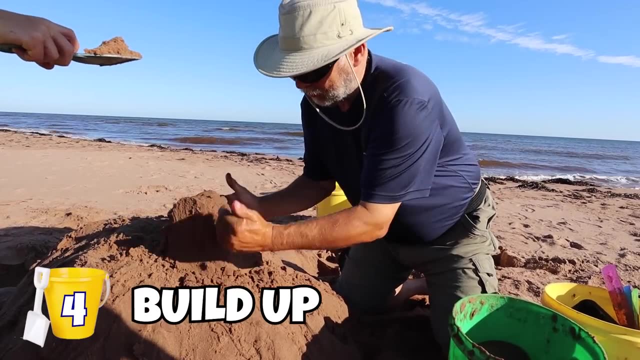 You see that mud. That's what we build with. You see how I'm building up. There's another block That's for build up. It goes like this: You cut at the top, You cut towards your hand so you don't lose parts. 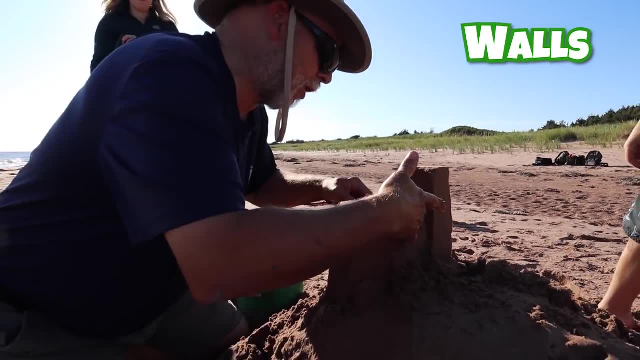 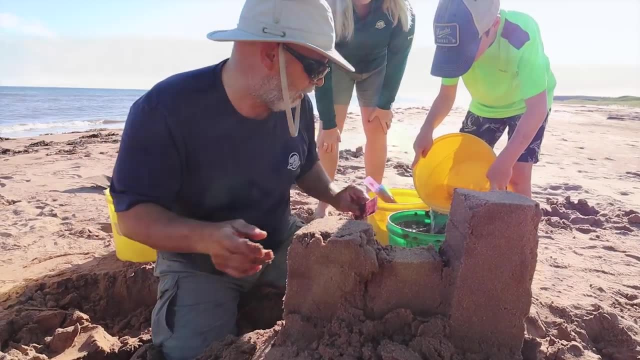 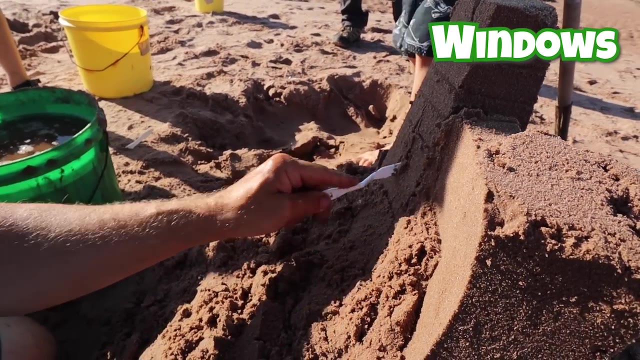 Step five: Sculpt, And then I'm making a wall. And you see I use the ruler just to trim. Yeah, Maurice uses tools like a ruler, palette knife and a putty knife. We can cut in, make a window. 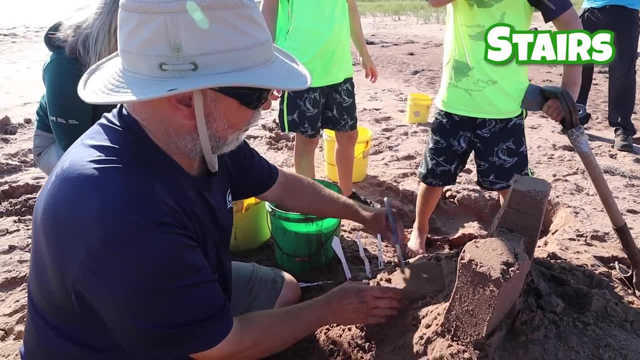 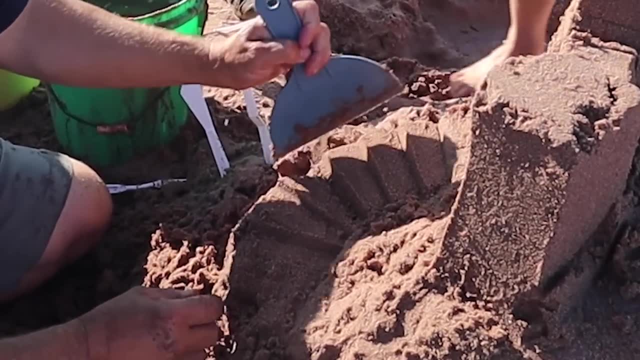 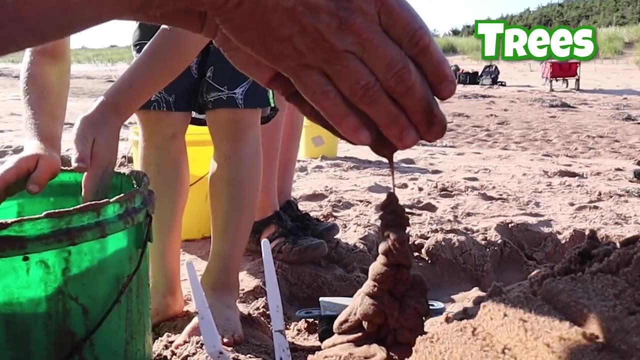 And then what you do is you go like this: Cut and slide, Cut and slide, Cut and slide, Staircase, Cool, We'll do some trees with that too. You see how I make the trees. I let the water drip off my fingers. 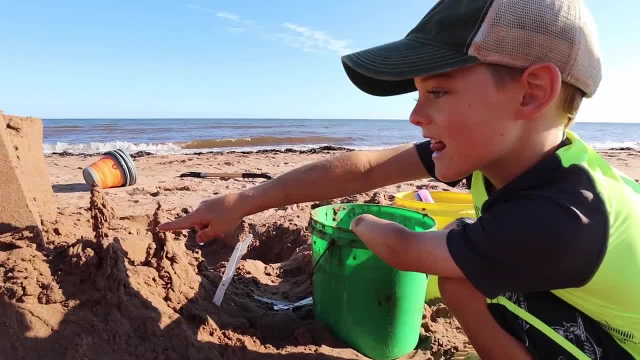 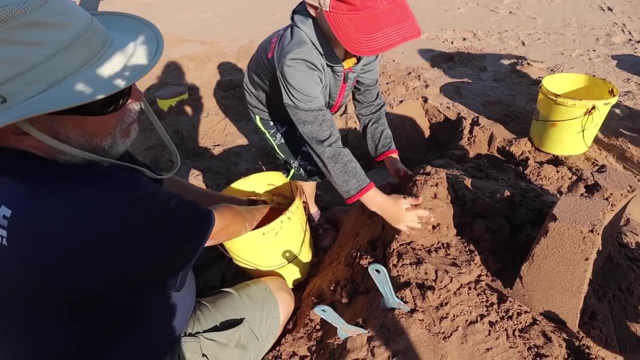 I made a really, really tall tree That looks pretty cool, With some branches. Yep, we're starting to get the hang of this. So the trick is, guys, the wetter sand better sand side and slide, And if you whack it, you crack it. 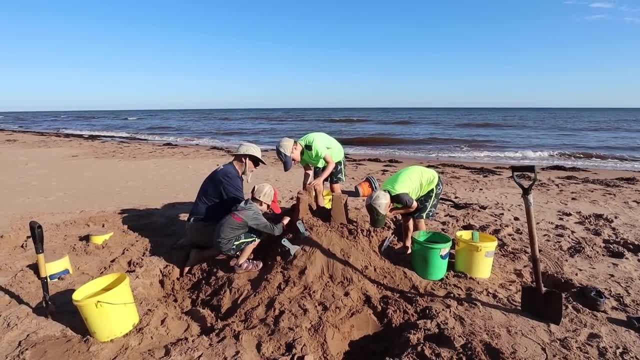 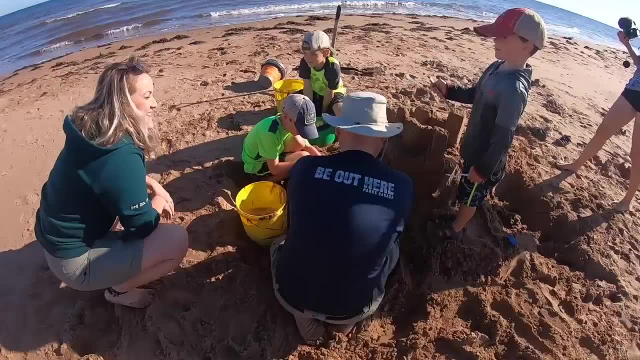 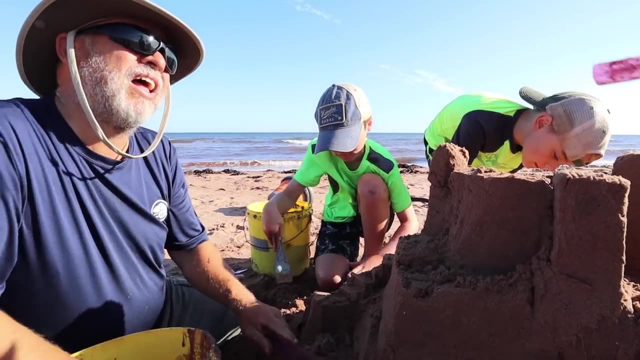 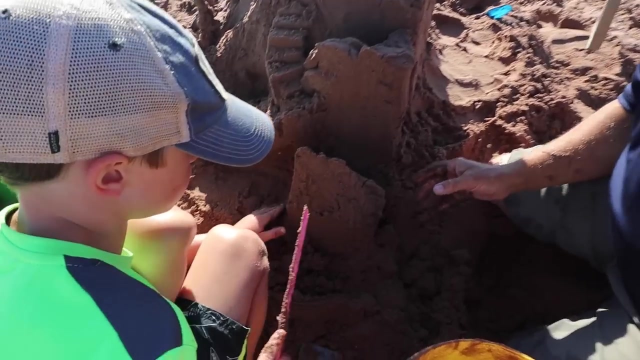 Oh yeah, We are making progress. Hey guys, it's me Wilder. It's time for the most important step. Use your imagination. I made little details on the top, So you're just taking your time and then it should work. 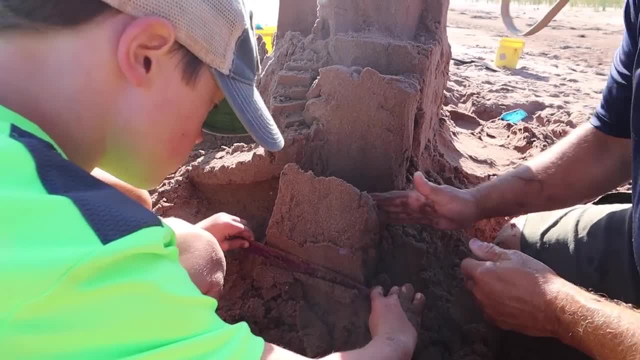 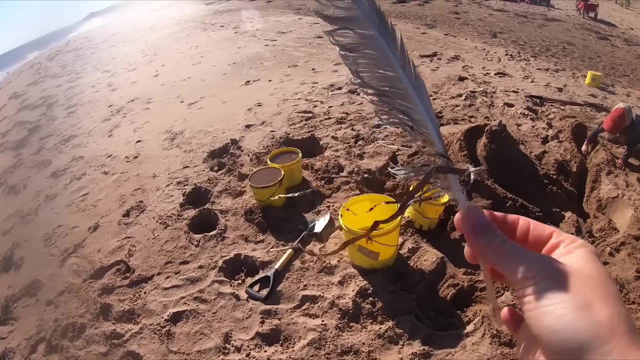 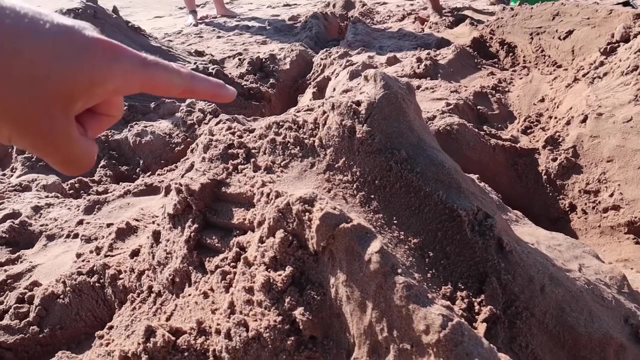 We'll just go like this, Like this: I made those trees And that bush, Archer. I have a present for you. Archer, what are you doing? bud Making balls, Nice, So the ball goes down through and in there. 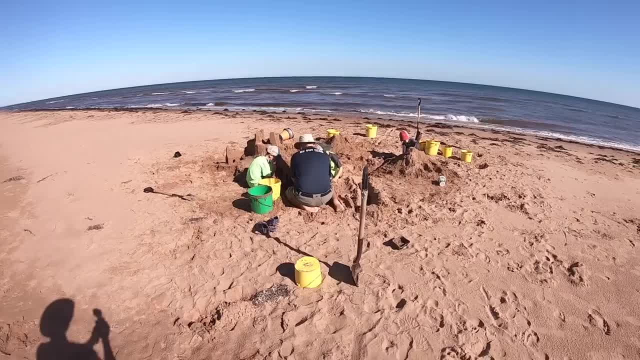 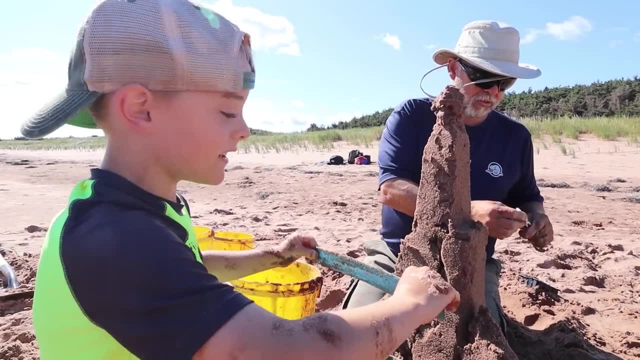 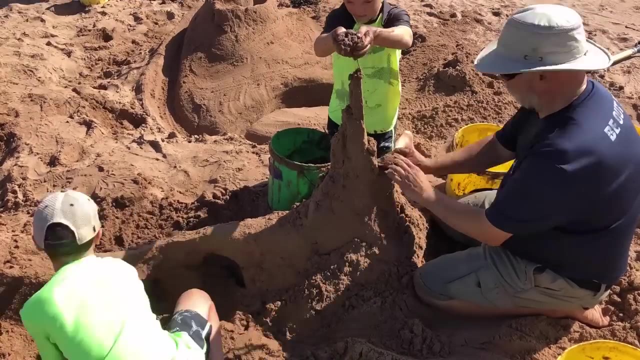 They have braces and the balls race down the hill. Yep, with Maurice's help, the castle is starting to come together. It's looking good. I'll just balance it right here. I'm building trees on top of the tower. Yes, sir. 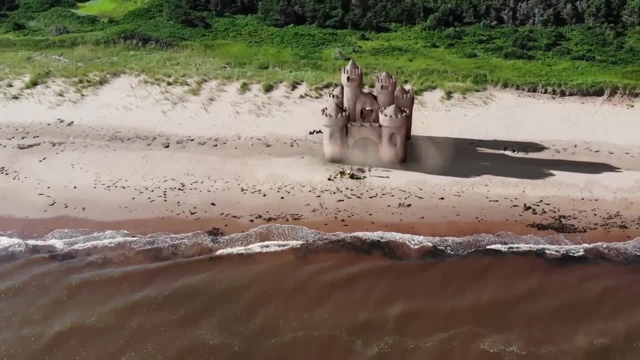 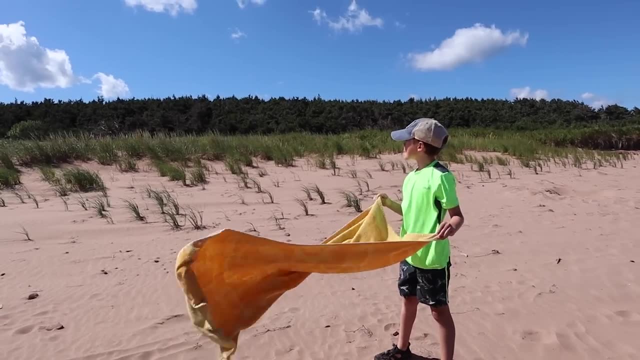 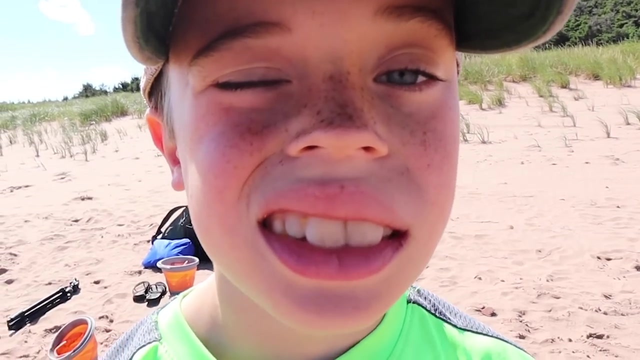 Our imaginations were running wild And our castle was getting so big You could probably see it from outer space. And back to reality: It's pretty windy Sand in the crackers. Okay, Maybe our castle isn't that big, But by the end 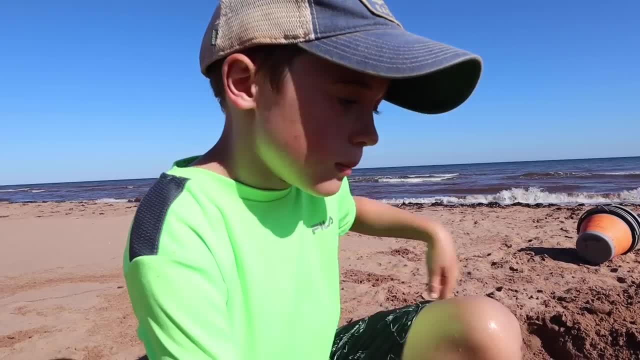 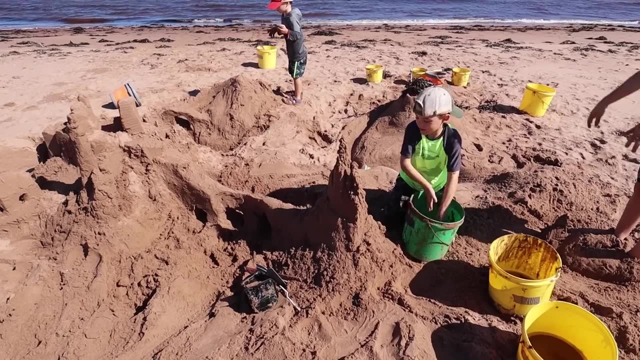 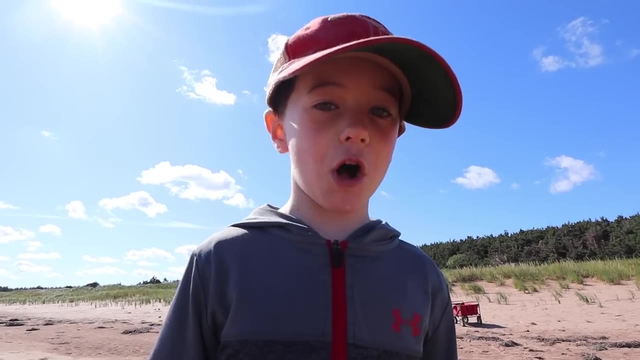 we each had something we were really proud of. I made this building and we made a hole through here and through here, and then I made the stairs. Look at the biggest tree. I made it from down here all the way to up here. It's a ball track. 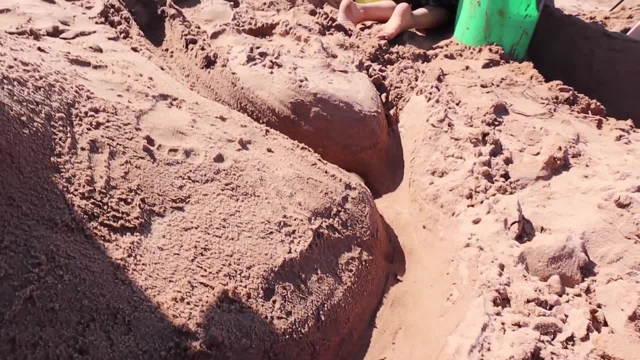 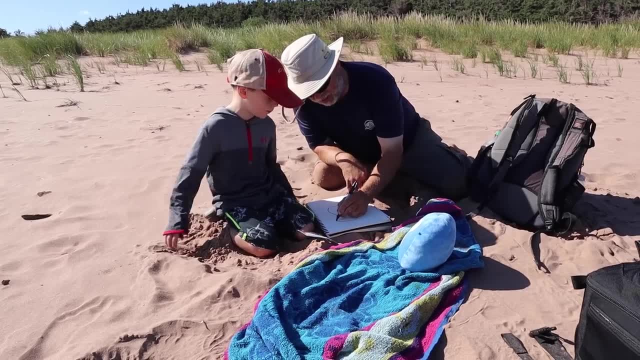 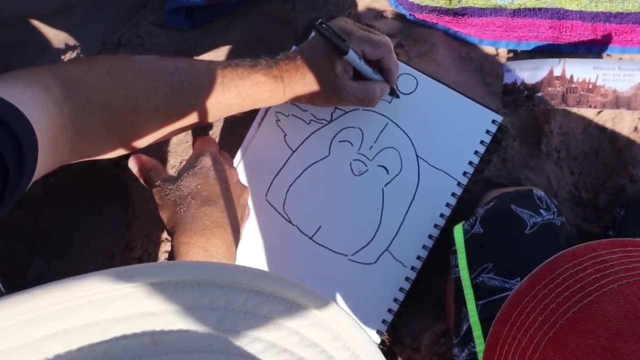 Nice, Let's see it. Here we go. Get rid of that. Did you have a good day, Archer? Yeah, That's good. Maurice is drawing my penguin. It looks like the blueberry sun is setting on us. You know what we should do. 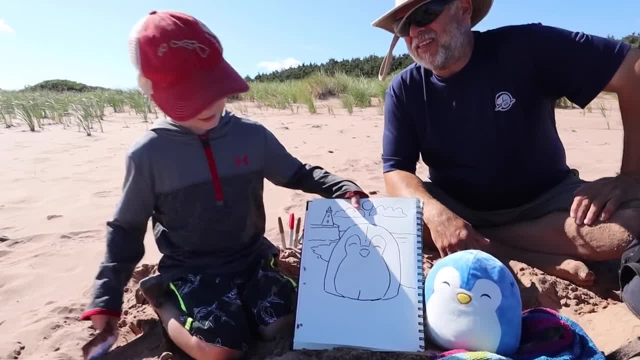 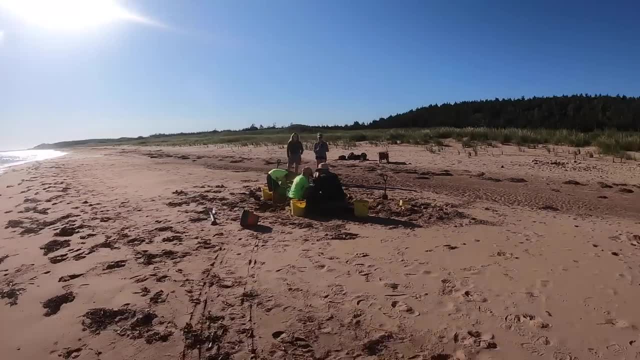 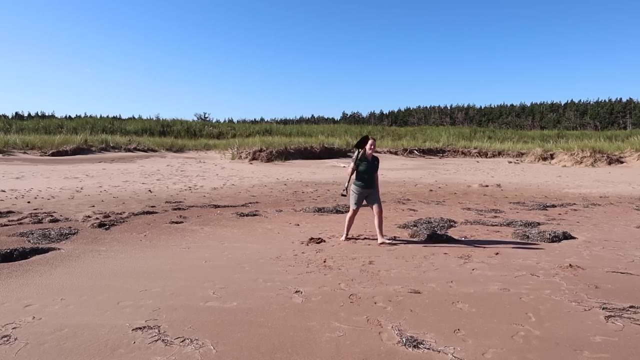 Oh, that's pretty special. Please don't forget to subscribe to our channel. Your subscriptions keep us going. So what do you say? Are you coming, Grab a shovel and let's get going.